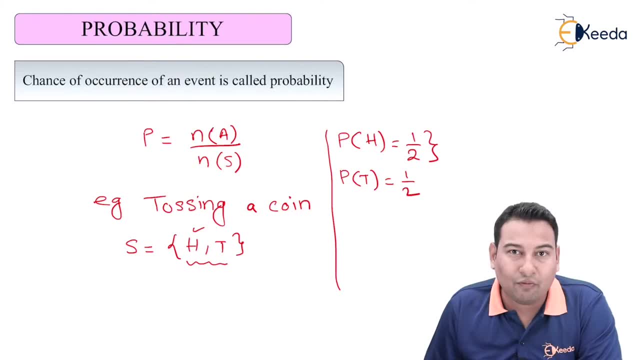 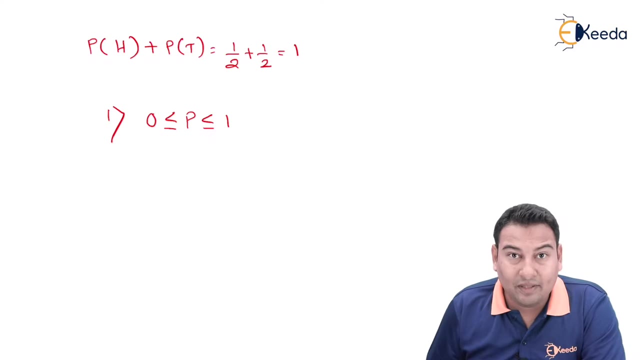 See here Individual Probability. That means Probability of head or Probability of tail. See here: it is half. So if you consider Individual Probability, it is between 0 and 1.. So this is the first point. So you might be thinking when will be the Probability 0?? 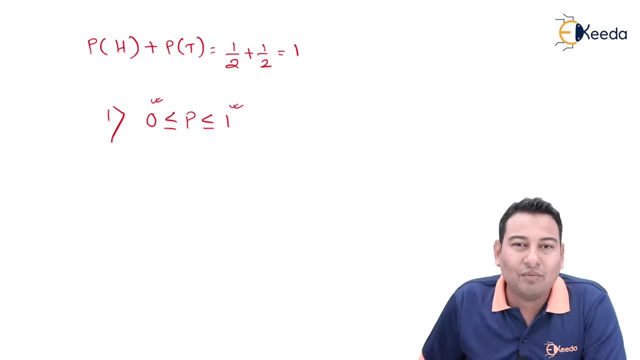 And when will be the Probability as 1?? Probability 0 means the event will never occur And Probability 1 means the event will surely occur. For example, if we have a coin and both side we have head. If we have a coin and both side we have head. 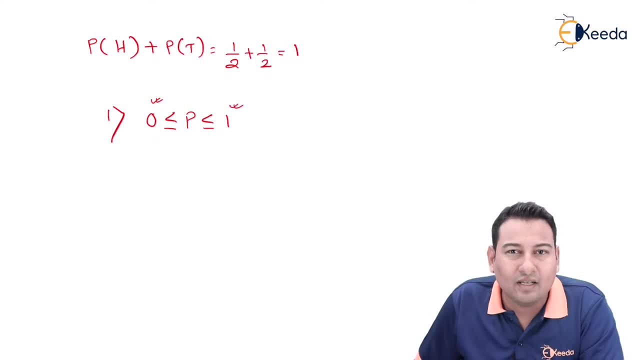 If it toss that coin, what is the Probability of head 1. Both the side head. So obviously head will come. That means event is going to occur, surely? So the answer is 1.. And both the side we do have head. 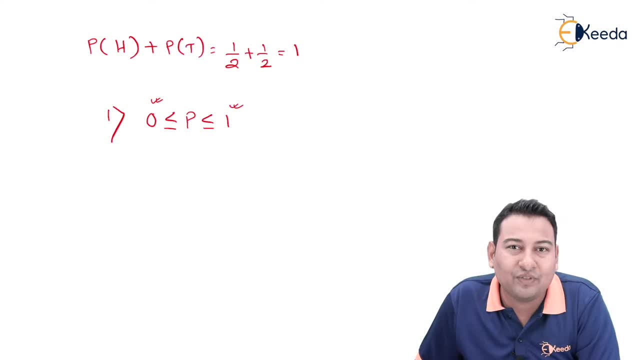 What is the chance of coming tail? 0. Tail can't come. Therefore the minimum Probability it can be 0. Event cannot occur and the maximum is 1.. The second point is: if you add all the Probabilities, your result is 1.. 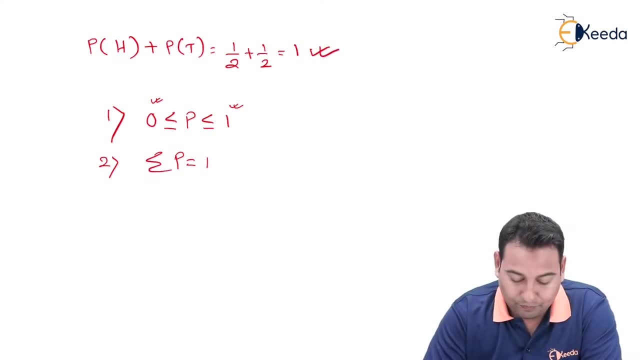 Summation of all the Probabilities is equal to 1.. See this: If you toss a coin, there are only 2 possibilities: Head or tail. Head Probability half. tail Probability: half. If you add, result is 1.. 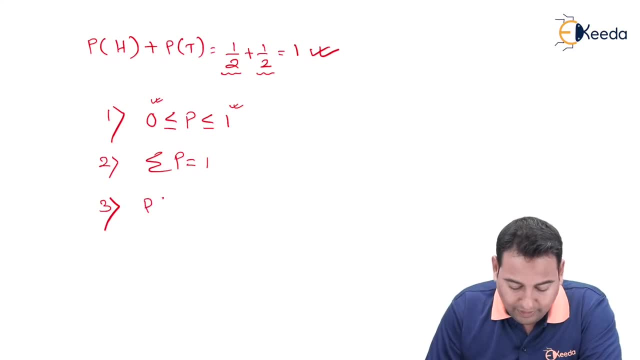 And the third point is Probability of occurring an event plus Probability of not occurring an event, The total is 1.. That means either the event is going to occur or it's not going to occur. If you add both the Probabilities, your result is 1.. 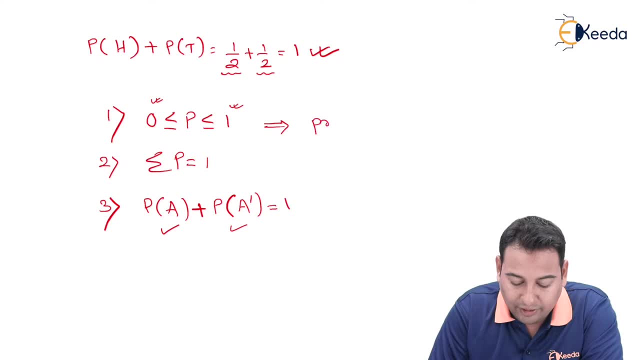 So from these points you can obviously conclude: Probability can't be negative. Probability can't be negative. We got it from this expression- only the first one, Because it is lying between 0 to 1, so it can't be negative. 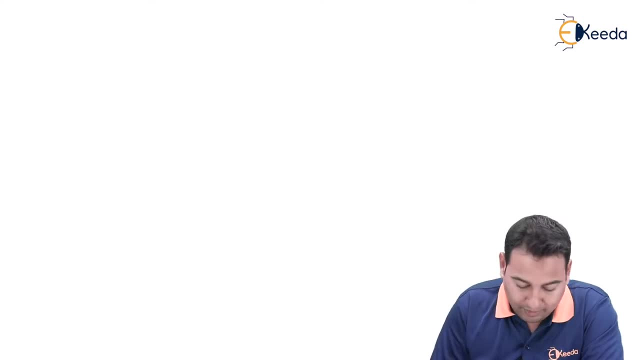 So let's confirm this point with the help of one more example. So let me take one more example: Throwing a dice. Can you friends tell me what are the possible outcomes if you throw a dice? So the possible outcomes in sample space S are: 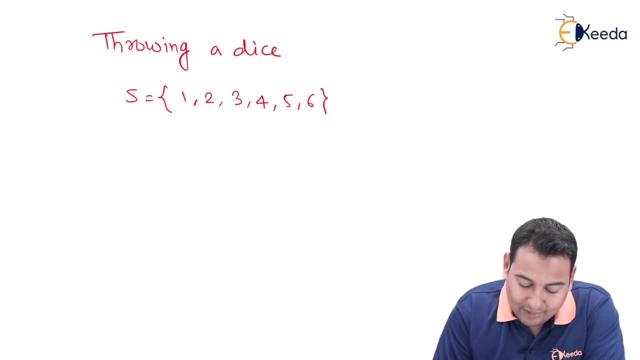 1., 2., 3., 4., 5., 6.. Again, if I'll check Probability of, let's say, 1.. What is Probability? How many times it has occurred out of total number of times? So 1 has occurred once out of 1,, 2,, 3,, 4,, 5 and 6.. 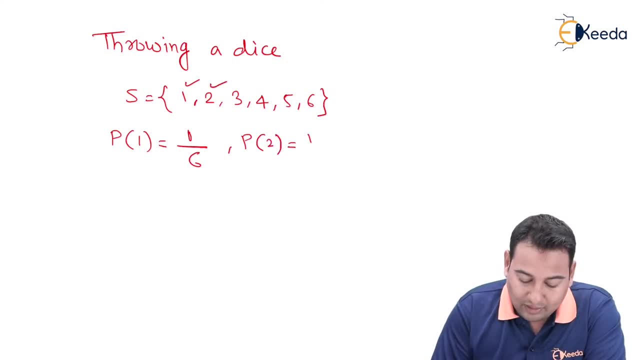 The same goes with 2.. Again, 2 has occurred once out of 6.. 3 is 1 by 6.. The same way, 4 is 1 by 6.. 5 is 1 by 6, and again 6 is 1 by 6.. 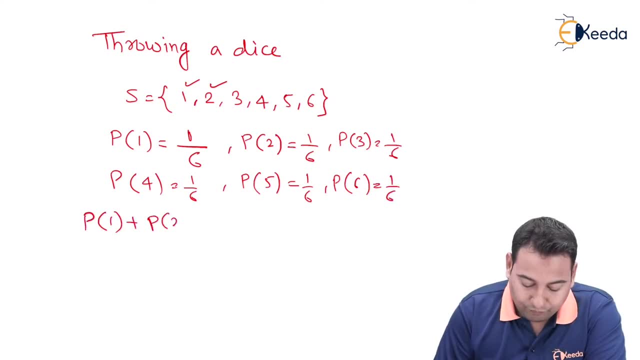 So if you add all the probabilities 1,, 2, up to 6, you will get 1 by 6,, 1 by 6,, 1 by 6.. If you add all the probabilities, your result is 1.. 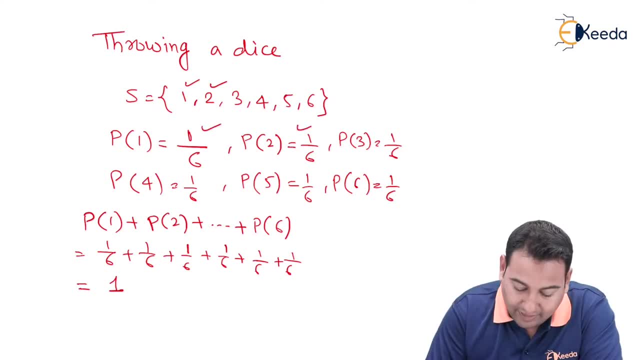 Again, both the points are verified. See your individual probability. Any event you check, it's lying between 0 and 1 and summation of all the probabilities is equal to 1.. So these are the two important properties, three important properties of probability. 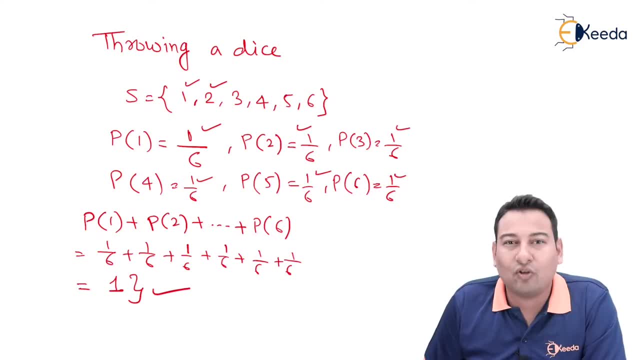 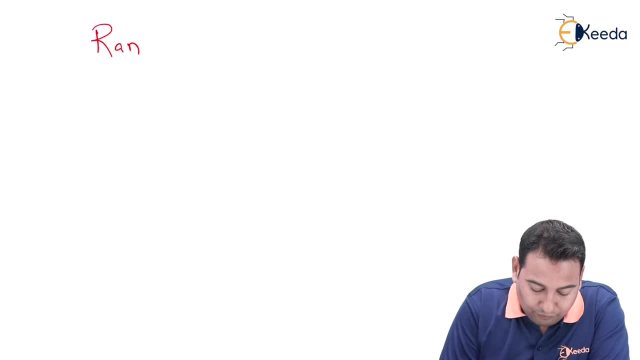 that you need to remember. Let's move on. This is the basic concept. This is the prerequisite for probability. Let's move on with the chapter. The first very important term is random variable. What do you mean by random variable? Assigning a number? there is a very complicated definition, but I'm giving you the simple. 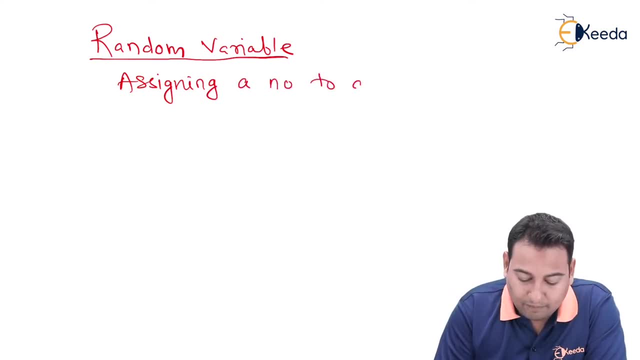 definition. Assigning a number to an outcome is called random variable. You might be thinking: what is random variable? Don't worry, With the help of example, I'll explain you. Let's say, tossing two coins. So, friends, can you tell me if I toss two coins? 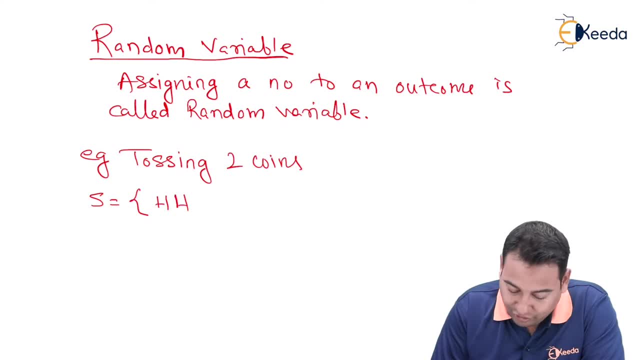 What are the possibilities? What are the possible sample space? It can be HH- HH means both the coins are having head. It can be HT, it can be TH or it can be T- T. Now let me assign a random variable. 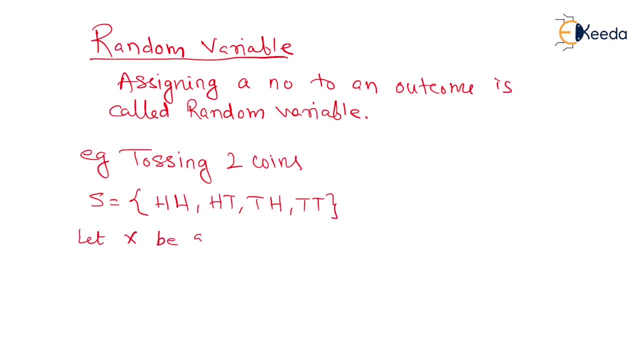 Let X be a random variable denoting number of heads. Is that clear? these are the outcomes. four: outcome h, h, h, t, t, h and t t. i am denoting, assuming x is a random variable denoting number of heads, i am assuming it x can be denoting number of tails. also that 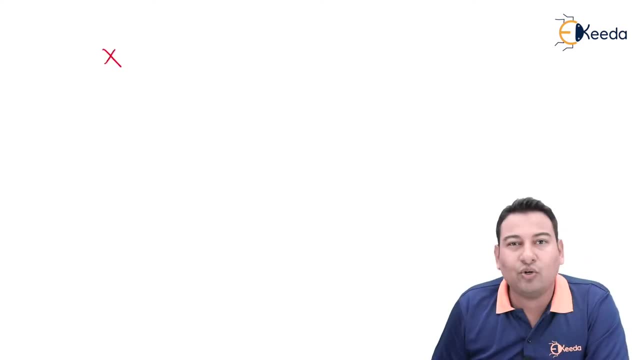 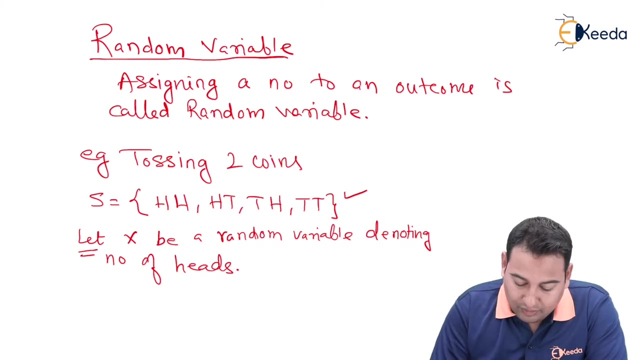 depends upon the problem. so x is the random variable denoting number of heads. so, friends, tell me how many heads are possible. looking at the example, you can say zero head. zero head means both tell one head, see here. and the maximum is two heads with the two coins. so number of 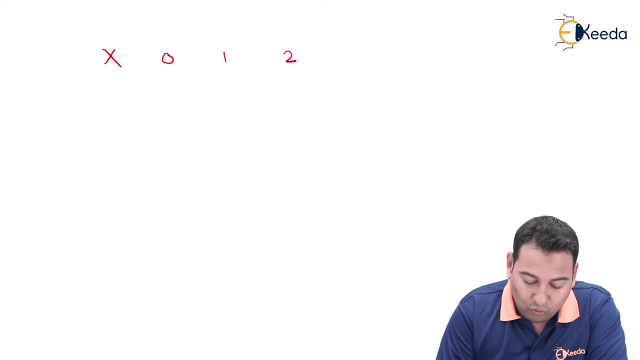 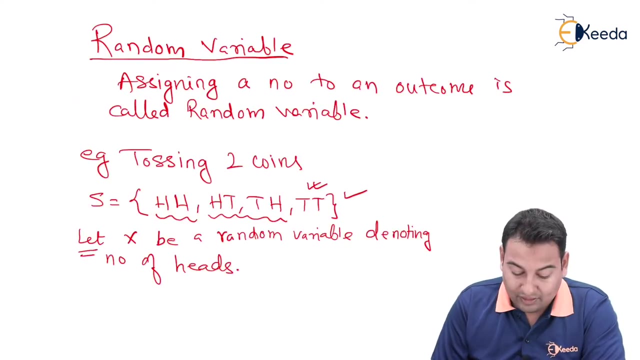 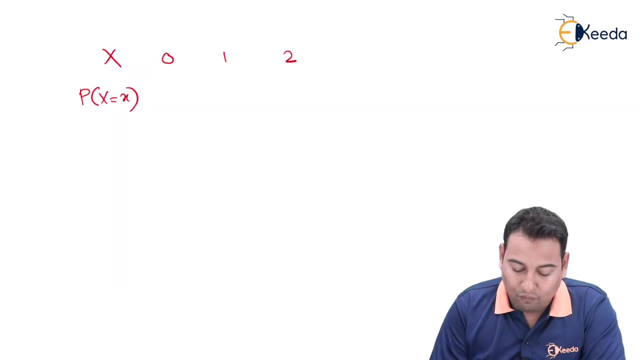 heads possibles are zero, one and two, and i am writing down this probability here. what is the probability of zero head? zero head means both tail, so both tail occurring one time out of one, two, three and four, so this is one by four. what is the probability of zero head? zero head means both tails, so both tails occurring one time. 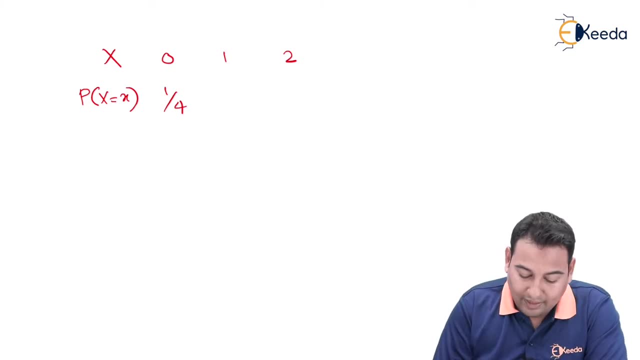 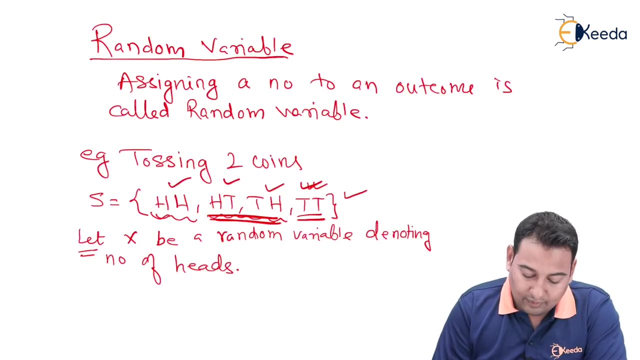 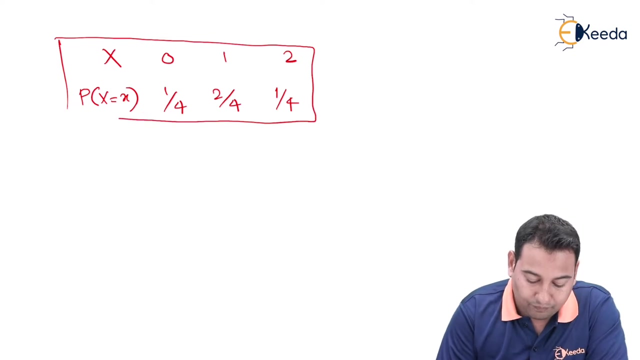 what about one head, one head occurring two times out of four and two heads- this is the term, two heads that is also occurring one out of four. so this is the table we are ready with. again, you can verify the point. individual probability lies between zero and one. 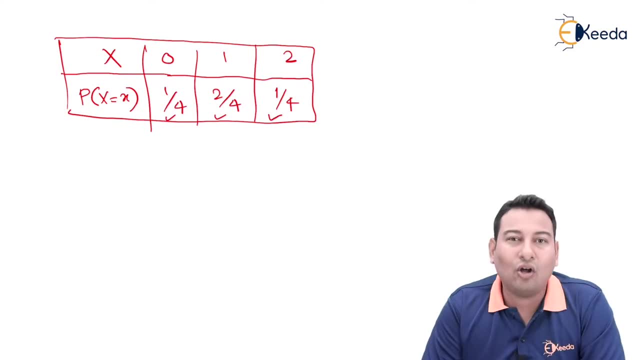 so see here: one by four, two by four, one by four, all are lying between zero and one, and some of them are lying between zero and one. so this is the probability of zero and one summation. if you add all this one by four, two by four, one by four, the answer is one. 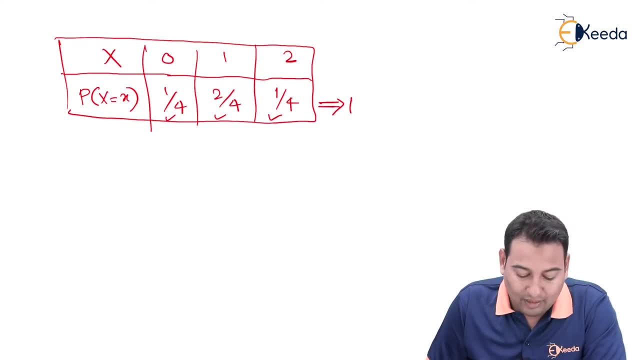 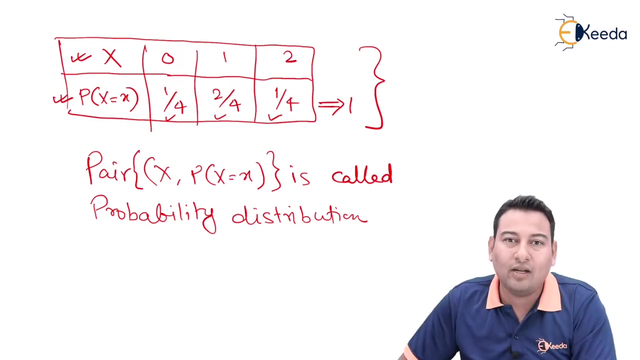 both the points are verified. this is your random variable x and this is the probability of random variable. this organization, that means the pair x, comma, p of x, is called probability distribution, which is one plane for knowledge, spacebild. so this is our chapter, actually probability distribution. so from the problem we're going to find it out: the x, that is random variable. 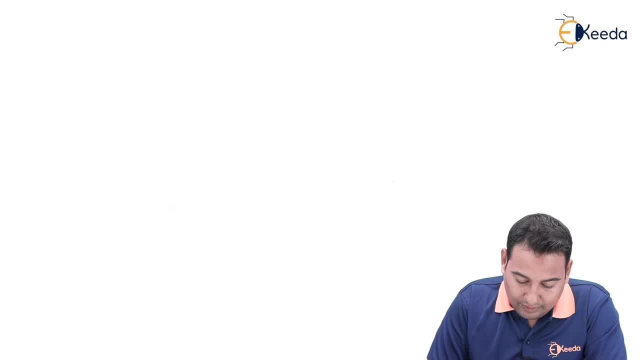 we're going to find it out its probability, and that pair is called probability distribution in our chapter. basically, probability distribution is of two moment zeros, one by four. so which is our probability distribution is of two types. one is your discrete distribution and one is continuous distribution. one question you will expect from this in the exam? for sure. 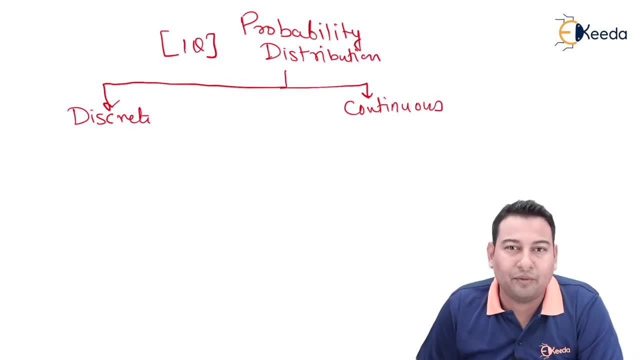 so prepare this table very well and one question is confirmed. first of all, what do you mean by discrete and what do you mean by continuous? discrete means you should have values, numbers, intervals. basically, you can say: interval means, let's say x, equal to, let's say 1. 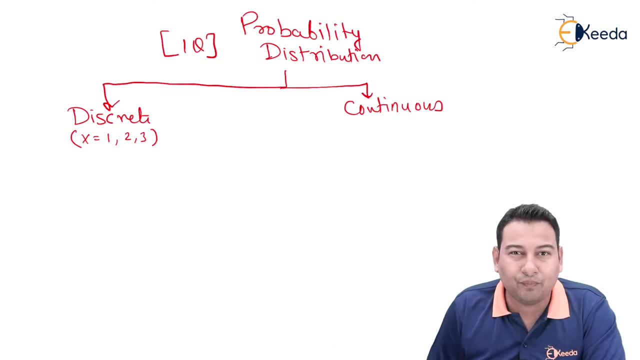 2, 3. so this is the example of discrete and continuous means, something like this: if i ask you, what are the points, how many points are there between 1 and 2, what is the answer? between 1 and 2, how many points are there? it should be infinite. this should be your answer. 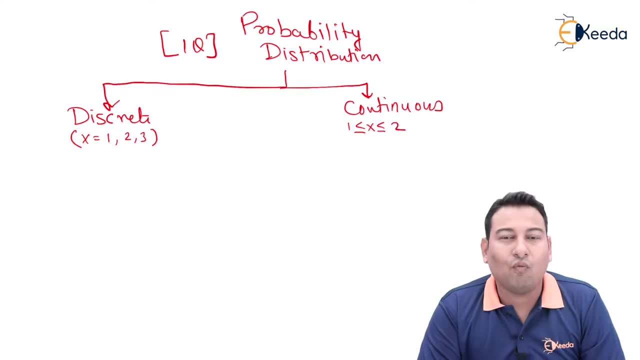 because let me give you example- 1.1, 1.11, 1.111, 1.112 and so on. so there are infinite points between 1 and 2.. discrete will consider it as an interval 1 and 2 only, but in case of continuous we're going to consider all the points. 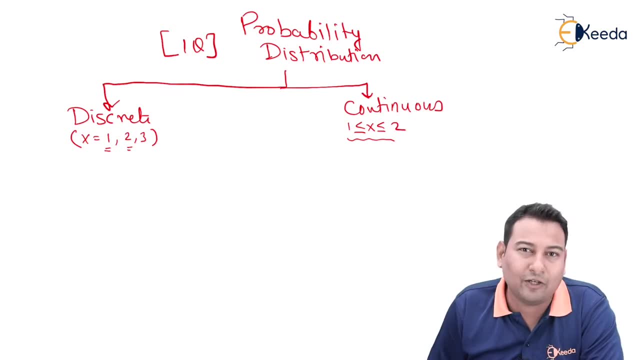 between 1 and 2.. so this is the basic difference between discrete and continuous. you should be very well prepared, with this table, to get 5 marks. so let us start the discussion. the first point is summation of all the probabilities equal to 1.1. 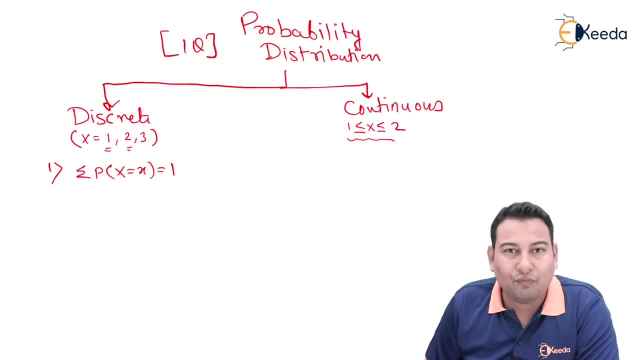 this is the first point in probability chapter. we write it as: p, capital x equal to small x. capital x means random variable. small x means a value of that random variable. for example, if the problem that we have discussed, capital x, can take value in case of tossing two coins, it can. 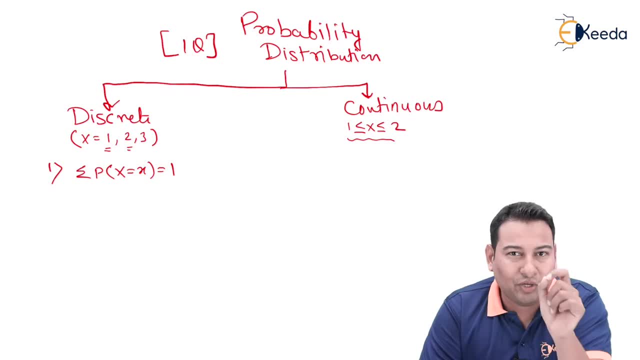 take 0, 1, 2 and small x means a particular value between 0, 1 and 2.. point number 2 is your mean, or expectation. mean is also called expectation. that is, e of x, equal to summation of x into px, where i am writing capital x, where i am writing small x. you should be very clear with that. 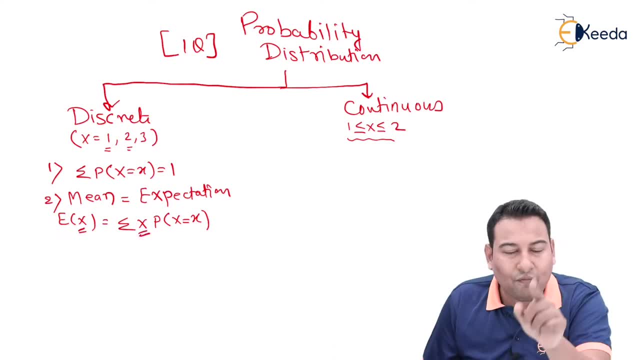 here we do have x, so therefore we do have x, e of x, x, p, x, x on both the sides. and the third point is variance. variance is e-x square minus e-x the whole square. so this is the formula for variance. now can you tell me, out of these two terms, which term is known to us? first one, second one, second one: 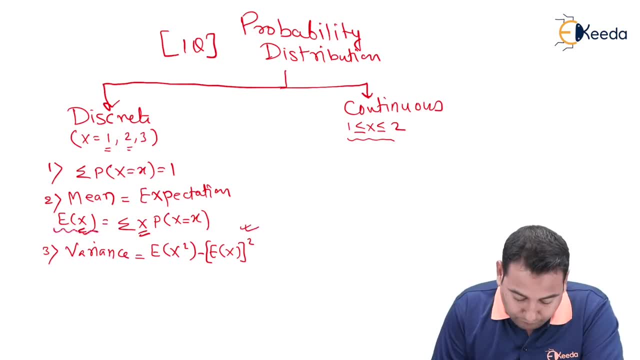 see, the second term is actually mean square, ex the whole square, that is mean square. so here one term is unknown, that is ex square. and the formula for ex square is is: when it was ex ex, we took x into px. So when it is ex square, we are going to take 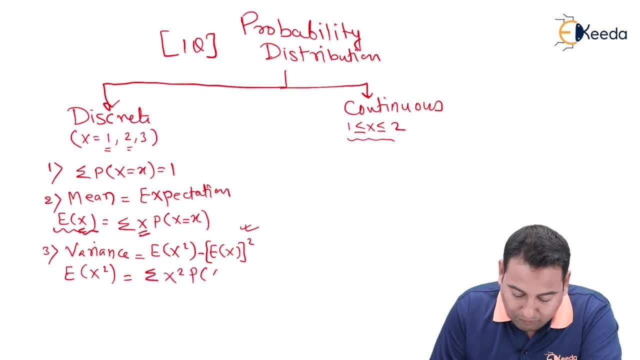 summation of x square into px. So remember this: When it was x, we took x. When it is x square, we are going to take x square. Probability will remain same. So this is a discrete part. Let us move on to the continuous part. The formula sequence will: 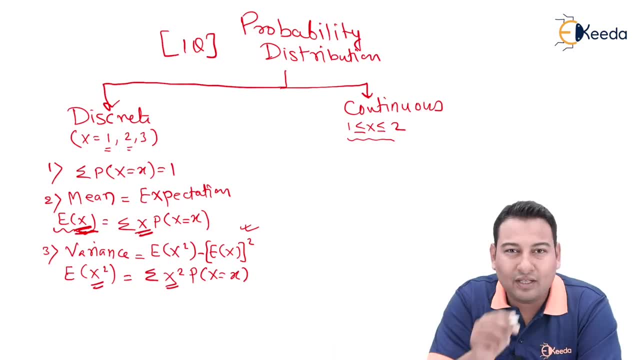 remain same. The only thing that you need to remember is, in case of discrete, we do have summation, But in case of continuous, the summation is replaced by integration. So here, the first is summation, that will be replaced by integration. first of all, 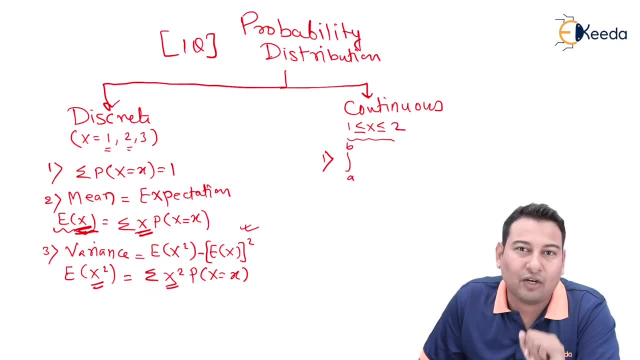 And the second thing is probability will be replaced by function. So that is f of x, dx. Two things clear. Summation will be replaced by integration and probability will be replaced by function. Next point: Mean equal to expectation e of x. E of x is summation of x into px. Summation will be replaced by. 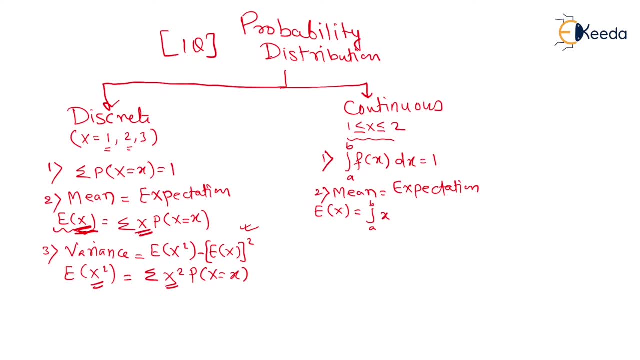 integration. X will remain as it is And p of x will be replaced by f of x- dx. This is my mean and expectation. Let us move on with the next formula, that is, variance. Variance basic formula is same: ex square minus ex the whole square. Again, the unknown term is: